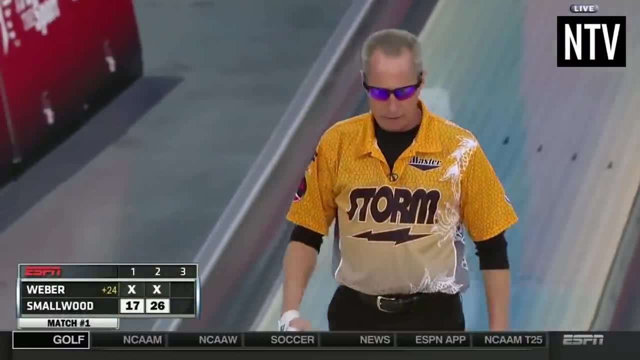 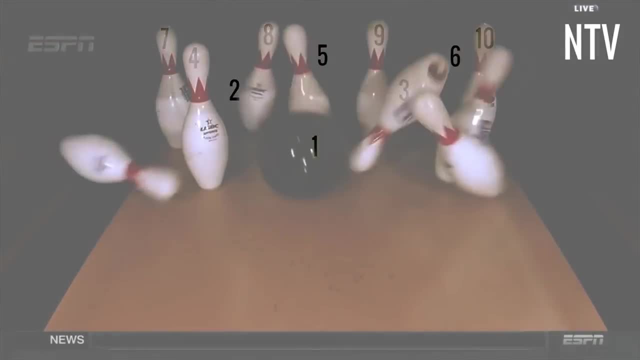 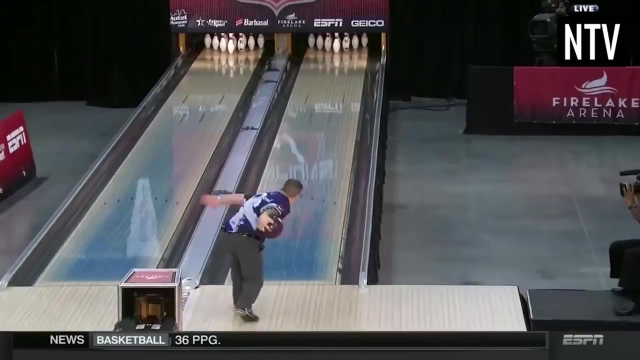 they land in the gutters and will be carried past the pins. The pins themselves are 15 inches high and are arranged in a triangle formation. Each pin is designated a number. A bowler uses a large, heavy ball and has up to a 15 foot approach to the foul line, which is the start of the lane. 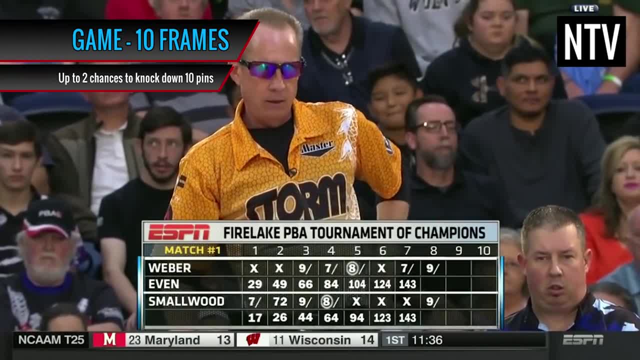 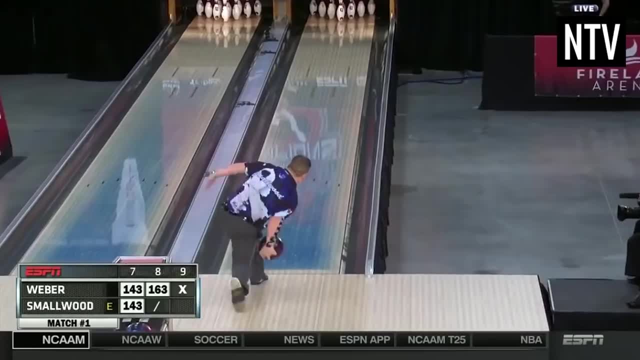 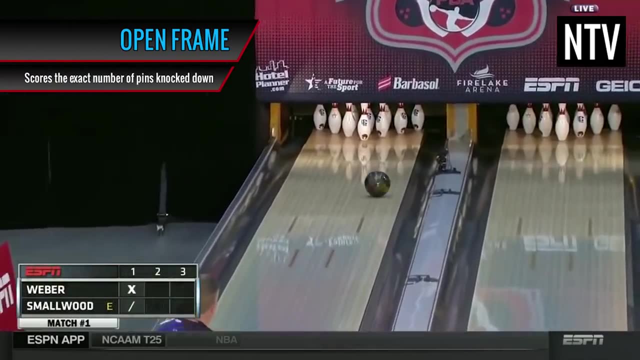 A game is divided into ten frames. Each frame represents one turn for the bowler. In a turn, the player is allowed to roll the ball up to two times. This means that you have two chances to knock down all ten pins. If you fail to knock down all ten pins with your two balls, this is known as an overhand. 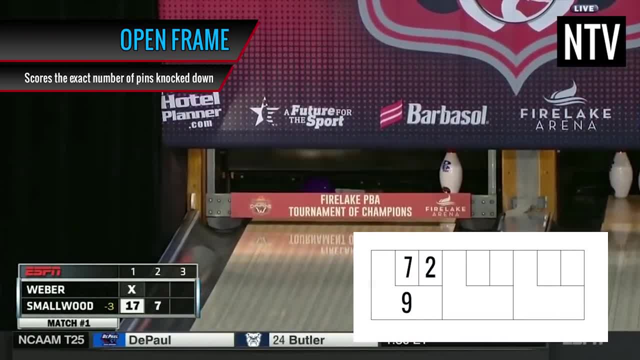 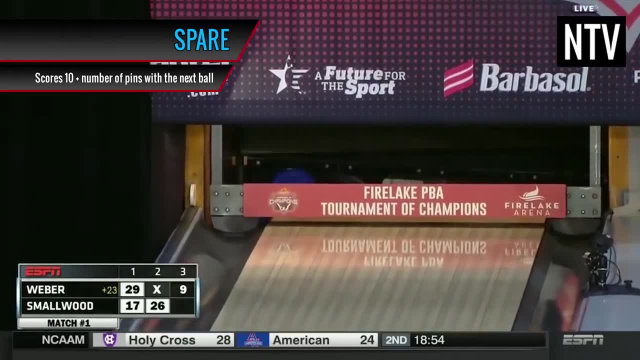 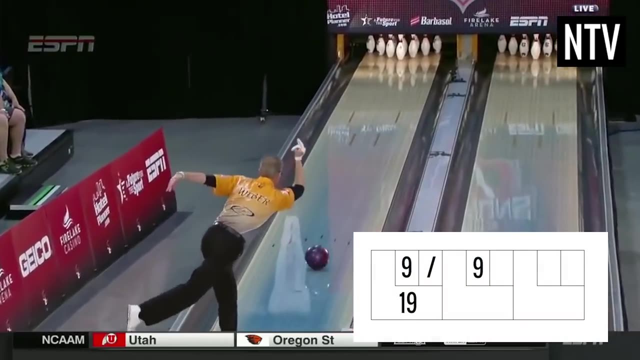 frame and this scores the exact number of pins that you knocked down. If you do knock down all ten pins with two balls, this is known as a spare, and this scores ten plus the number of pins knocked down with the next ball. For example, if you score a spare and then with the next ball score nine, the spare frame. 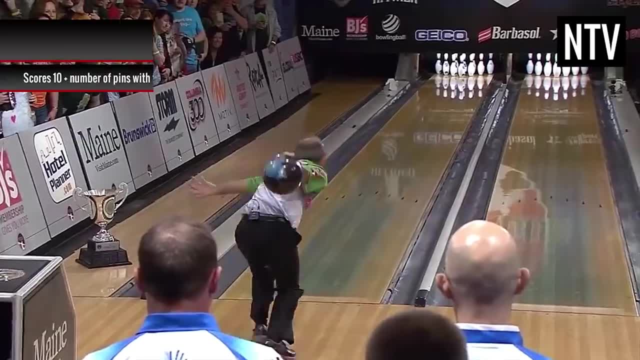 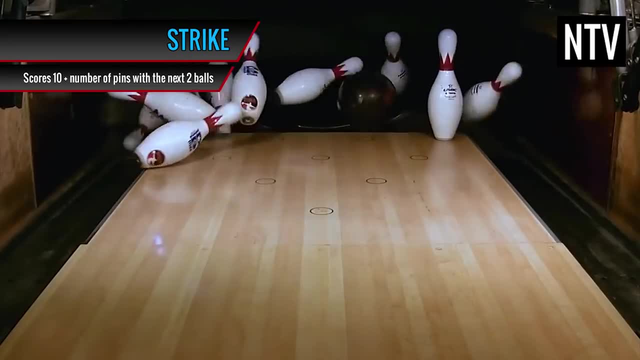 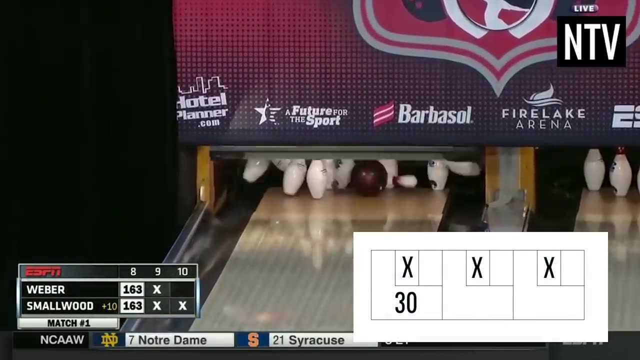 is ten plus nine, which is nineteen. And if you knock down all ten pins with your first ball, this is known as a strike. This scores ten plus the number of pins that you knocked down with your next two balls. For example, if you score a strike and then follow it up with another two strikes, the 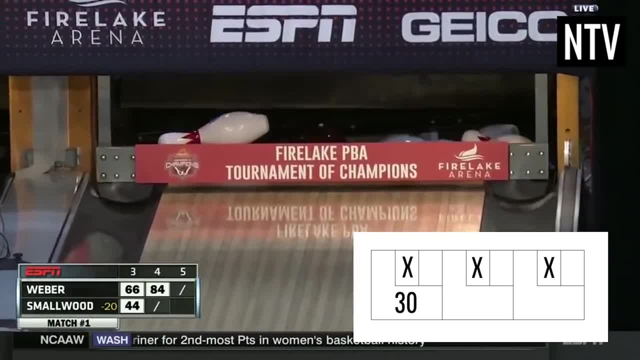 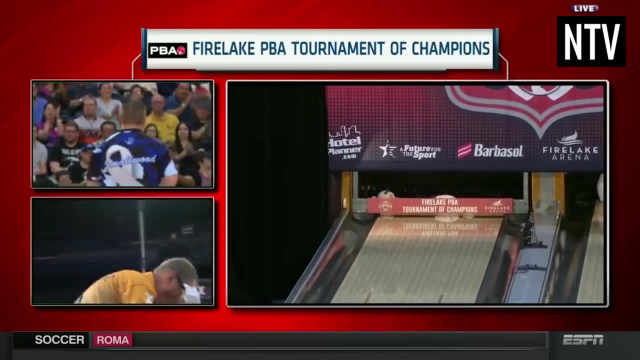 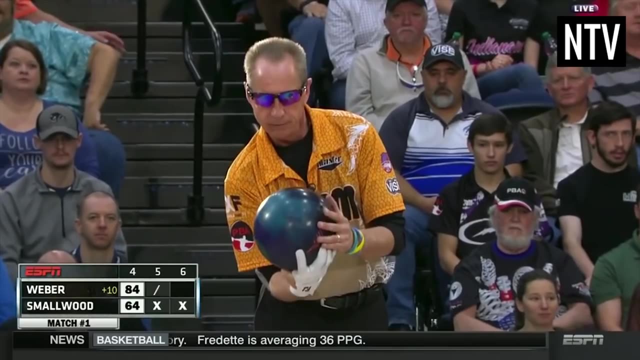 first frame is scored as ten plus ten plus ten, which is thirty points. Players generally alternate turns between frames and once both bowlers have finished ten frames each, the person with the highest score wins. Simple right. So why do they bowl the ball? funny? The whole idea is to maximise your chance of 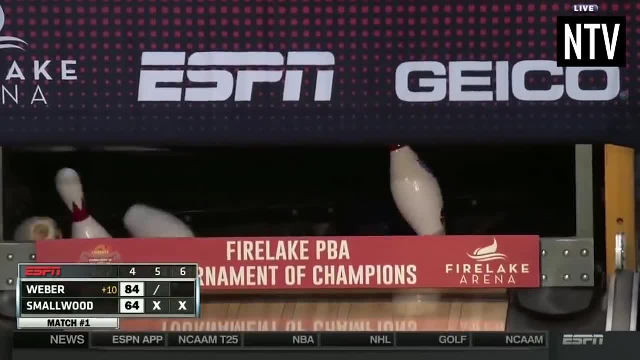 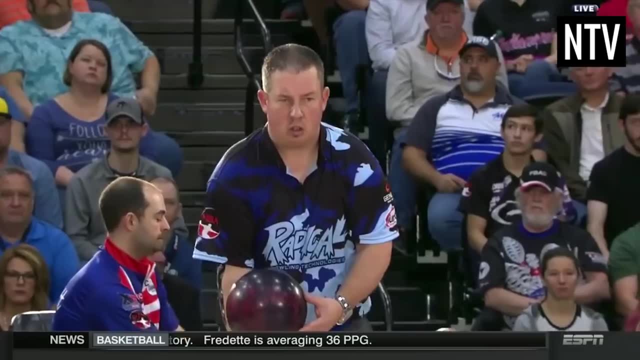 getting the ball. Players will start scoring strikes by hitting a certain section of the pins. This section is known as the pocket and this scientifically gives you the best chance of getting a strike. Therefore, bowlers will try and curl or hook the ball into the pocket. 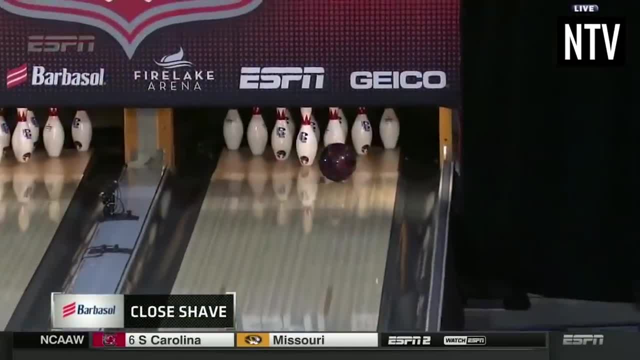 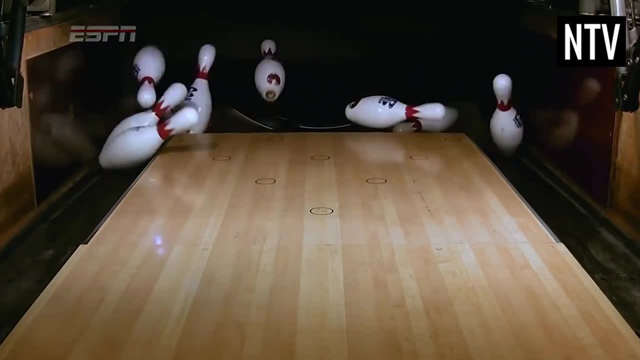 The lanes have oil on them that gets drier as you get closer to the pins, So players take advantage of that by throwing the ball at an angle with spin. in order to get the ball to hook into the pocket, They will use the triangular markers on the pins. 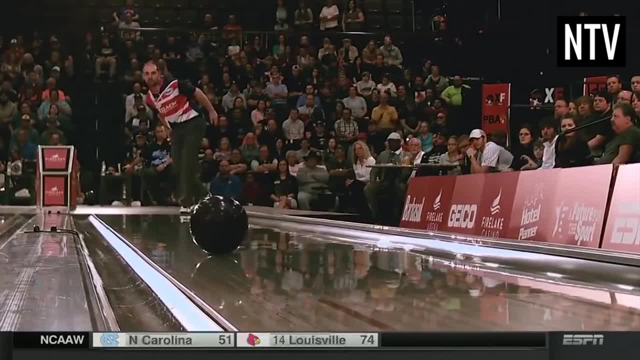 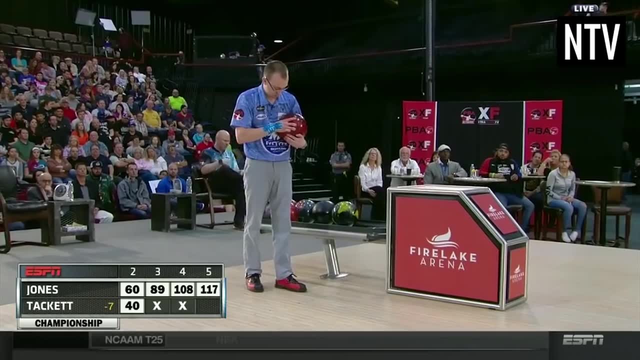 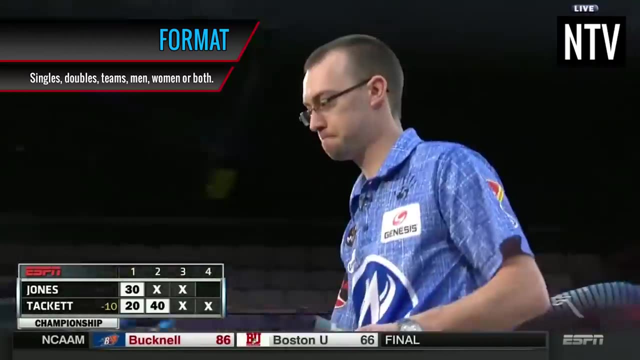 That's the bare basics of ten pin bowling, but there's a few other things you need to know before playing or watching a game, For example… Format. The most common format is a single match, where one person plays against another person, But there are also competitions for teams of two, three or four players to bowl against. 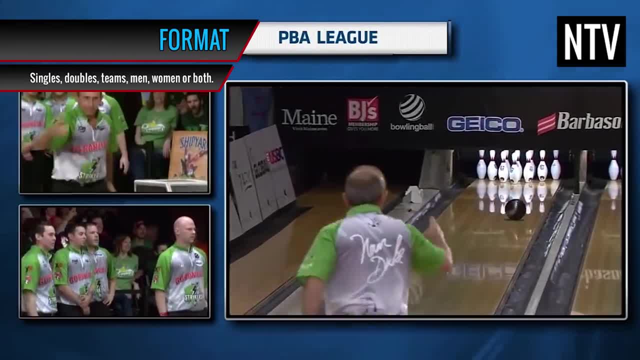 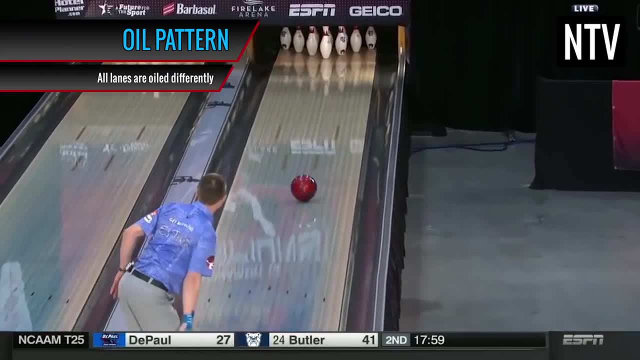 another team. There are separate contests for men and women, or a mixture of both: Oil, Oil, Oil, Oil, Oil, Oil Oil. Each lane is oiled different And, depending on the pattern, this dictates whether the ball will hook or not. 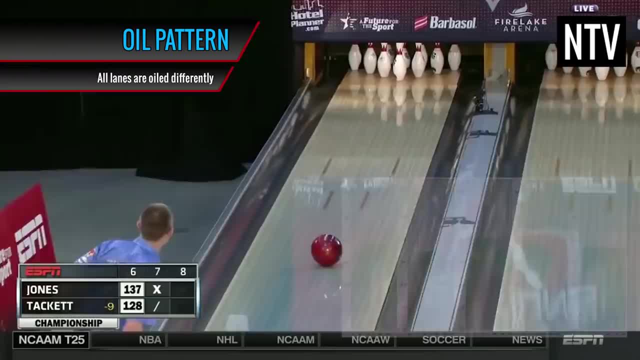 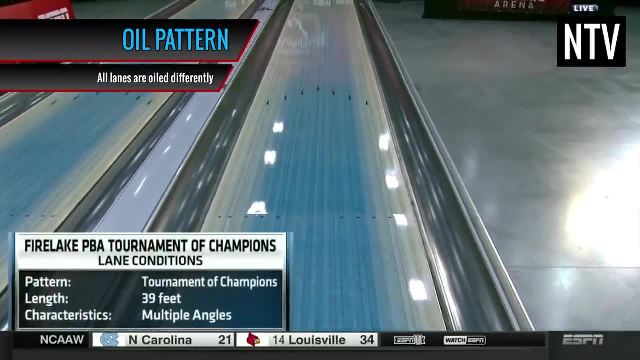 This is known as the oil pattern, and it might be helpful to check the oil pattern of the lane you're bowling on. In professional tournaments such as the PBA, they will add a blue die to the oil so that players and spectators can see where the oil is and where it's running dry. 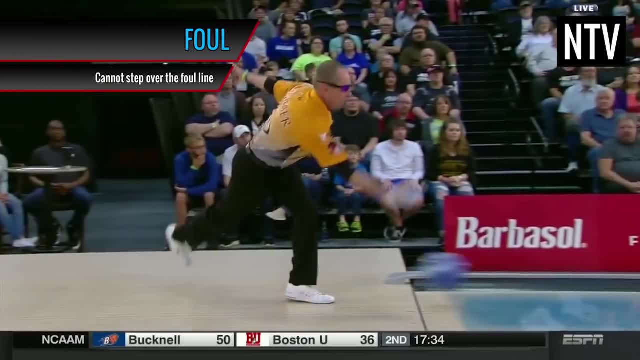 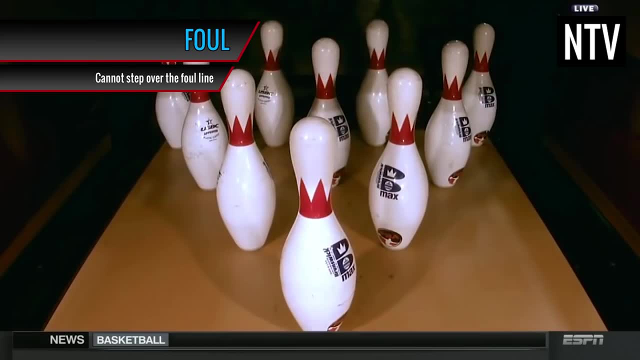 Foul. A player must not step or slide across a foul line when bowling a ball, So it shouldn't happen every time you are bowling a ball Foul –. doing so will count as a ball, but will not score. The pins that are knocked down are replaced. 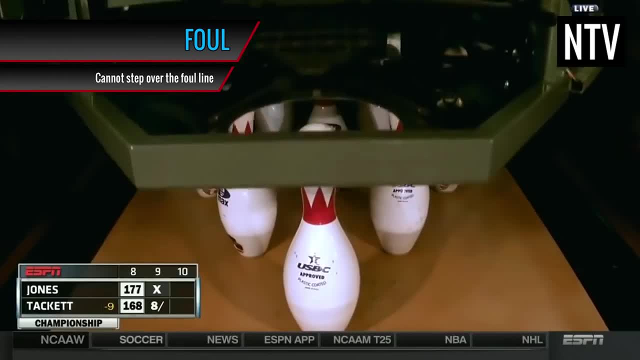 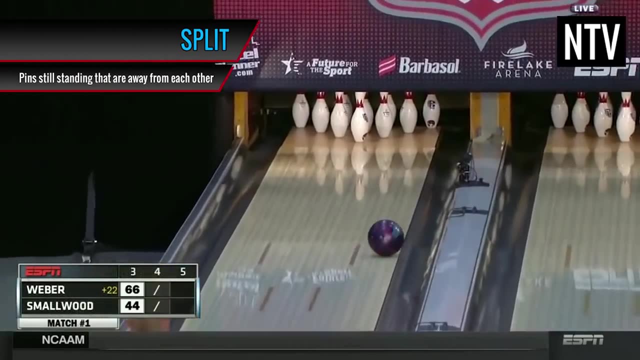 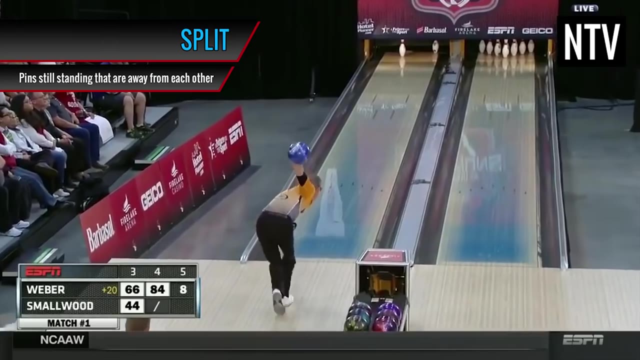 Also, any pins that are knocked down by a ball in the gutter or by bouncing off the rear cushion don't count either. Split – this is where the first ball of a frame results in pins away from each other still standing. To knock both pins down with only one ball left is difficult. 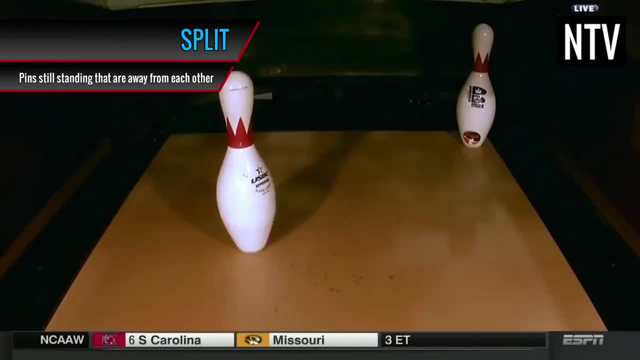 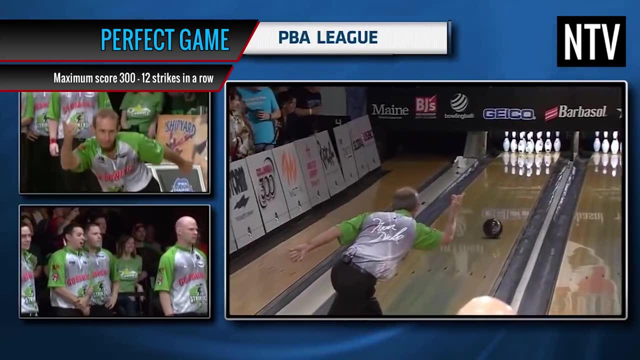 This is known as a split. Difficult but not impossible. Perfect Game –. in a game of bowling, the maximum you can score is 300 points. This is done by rolling 12 strikes in a row. Why 12 strikes instead of 10?? 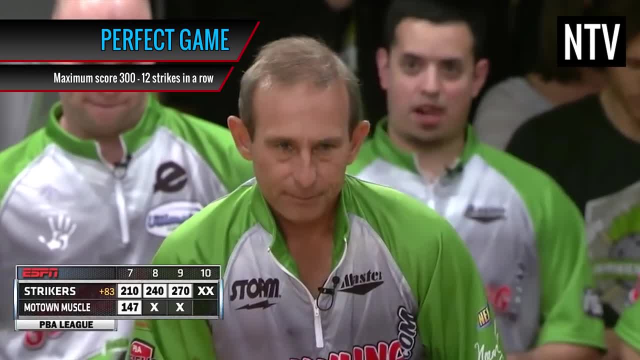 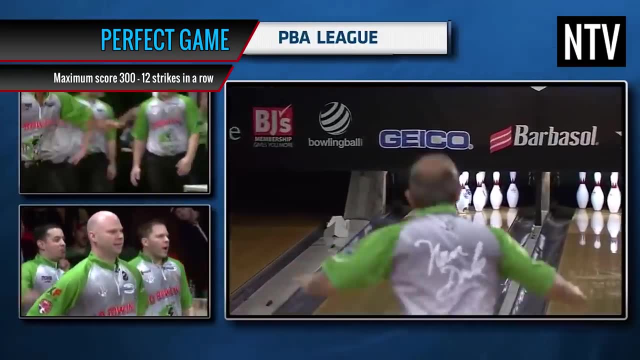 Because if the bowler gets a strike in the last frame, the score of that frame cannot be recorded before rolling twice more. This is known as a perfect game, or a 300, and is the equivalent of a 1-4-7 maximum break. 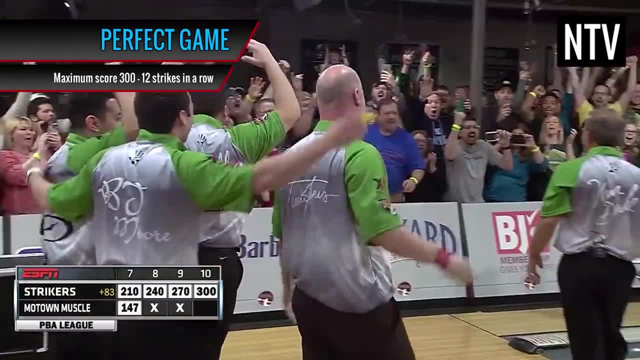 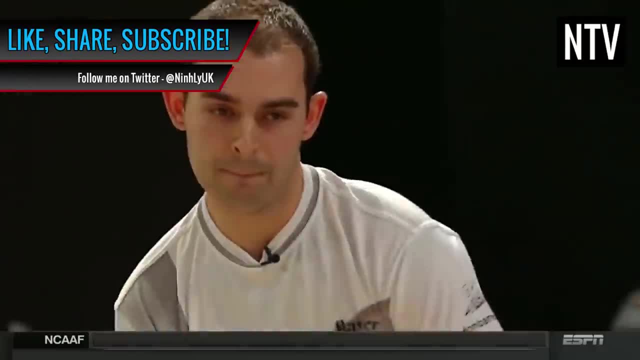 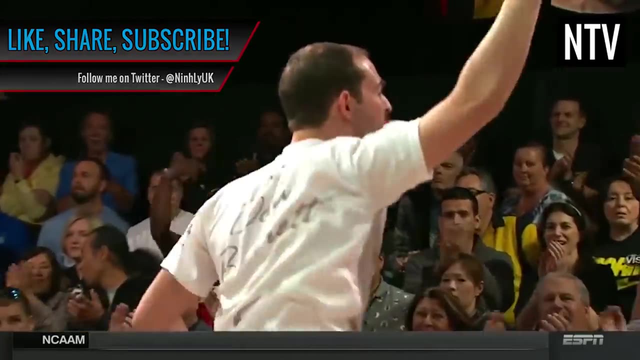 in snooker and a 9-dart finish in darts. As you can tell, it's not easy.